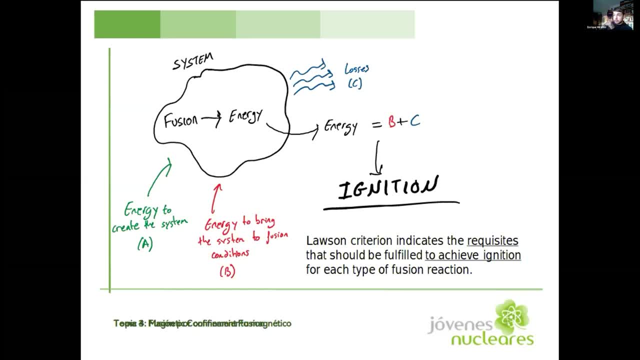 This means that the energy produced in the system itself makes the reactions self-sustained. So we don't need to bring energy to the system to bring it to fusion conditions, because the fusion reactions themselves are doing that job for us. So the Lawson criterion tells us what are the requisites that should be fulfilled to achieve ignition for each type of fusion reaction. 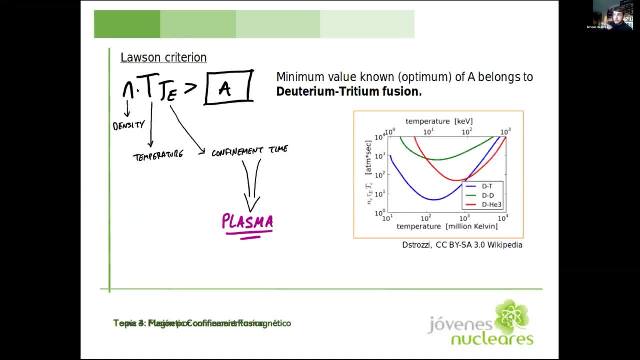 This Lawson criterion is a triple product of the density, the temperature and the energy confinement time, and this product has to be greater than some value a, And we know this. value a is the value of an energy content of this value a. 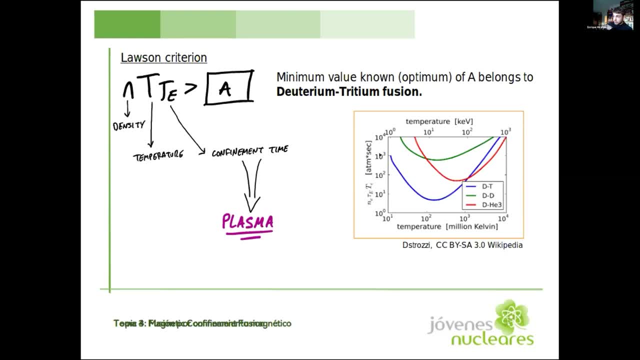 And we know this value. a is the value of an energy content minimum for the deuterium tritium fusion reaction. That's why we aim to make deuterium tritium fusion, because it's the easiest one. So we need to make this product large enough. We know some methods to increase the density. We know 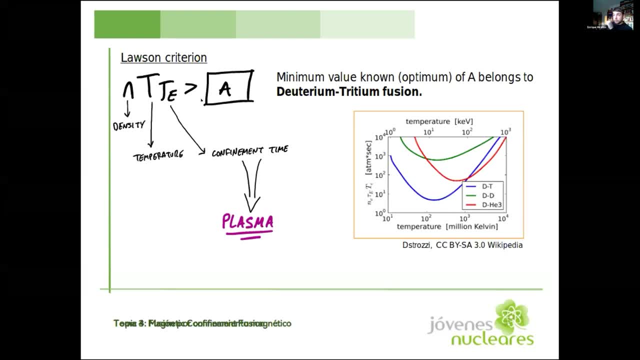 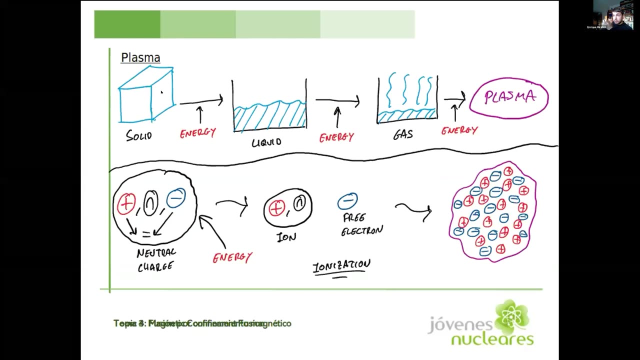 some processes to increase the temperature, But how do we increase the energy confinement time of a system? That's a bit trickier And we take advantage of the fourth state of matter, which is called plasma, To understand what plasma is. let's imagine we have a solid And we heat up the 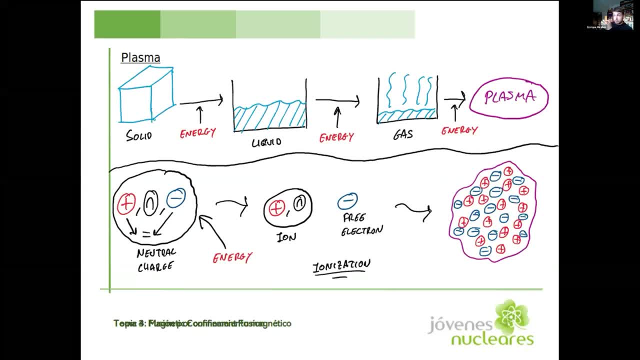 solid providing some energy. Eventually, the solid will melt and we turn into liquid. If we keep providing energy to the liquid, it will start boiling and then turn into a gas. And what happens when we keep providing energy to the gas, when we keep heating the gas? 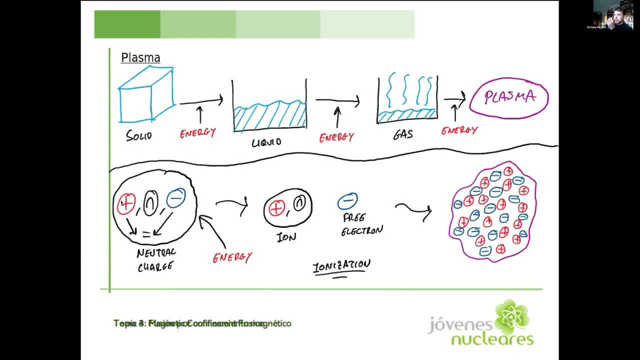 is that we eventually will achieve plasma. To understand this, we know that atoms are usually composed of protons, neutrons and electrons, And when the number of protons equals the number of electrons, we say that the atom is neutrally charged. It has neutral charge Because the 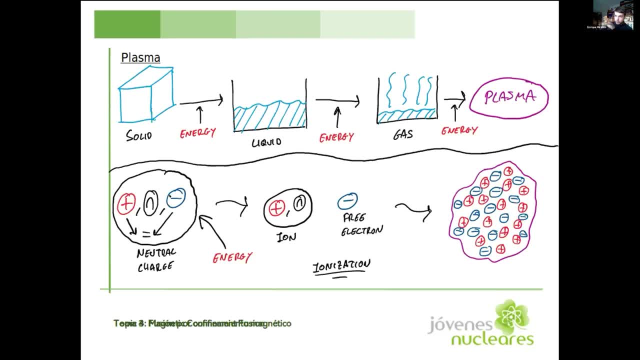 positive charge of the proton is being compensated with the negative charge of the electrons. But when we provide energy to this atom, eventually, what might happen is that the electrons might leave the bounds of the atom, And then we will end up with a pair ion-free electron. This process is 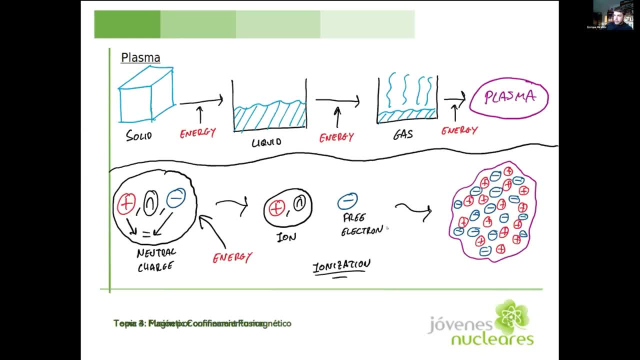 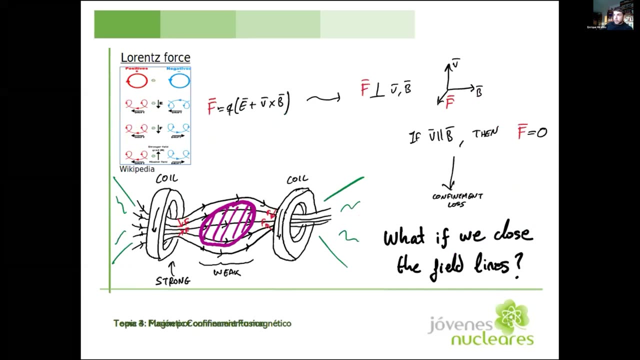 called ionized gas, And that's why plasma is also usually called ionized gas, Because it's like a gas where electrons and ions coexist independently like separate particles. The trick comes when we know that the charged particles feel a force when they are under the effects of a magnetic 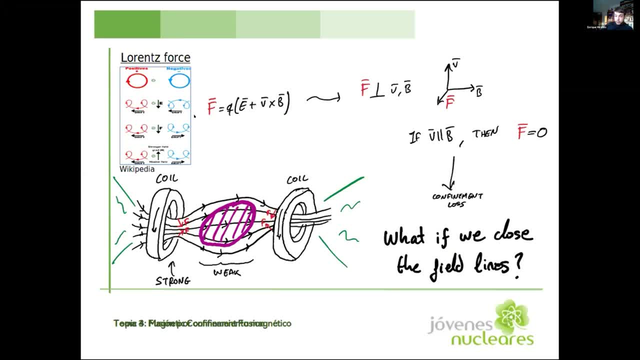 field. So we can use magnetic fields to exert some forces to the charged particles. This Lorentz force is perpendicular to the velocity of the particle and the magnetic field. So the early idea was to make this sort of magnetic bottle. it was called magnetic bottle. 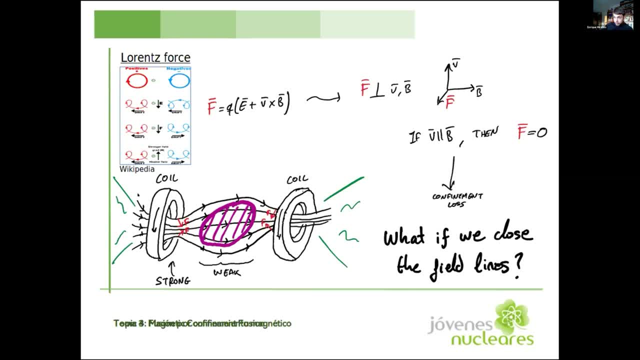 with two parallel coils. These coils will generate this magnetic field. It was stronger as we move close to the coil and then weaker in the middle, And the idea was to confine particles in the weakest region of the of the bottle, Because when the particles try to escape, 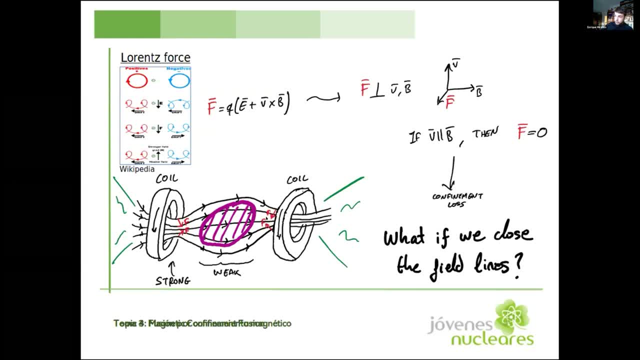 this way or this way they felt this Lorentz force that is perpendicular, And then the particles eventually bounced back to the middle of the bottle. But the problem is that when the velocity of the particle is completely parallel to the magnetic field, then this particle is not. 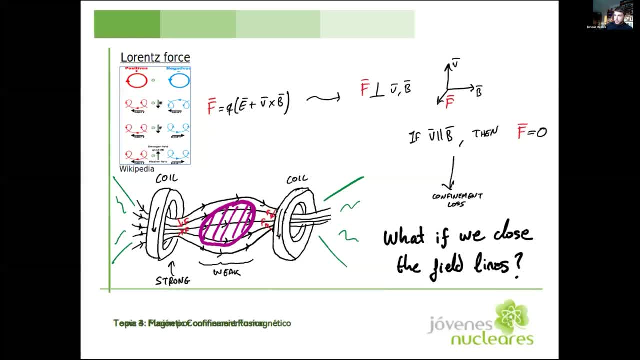 going to feel any force and then they could escape. So we have some kind of confinement loss here, because the particles that have a very large velocity parallel to the magnetic field then might escape this confinement. so they thought, okay, um, let's close the the magnetic field lines and let's make 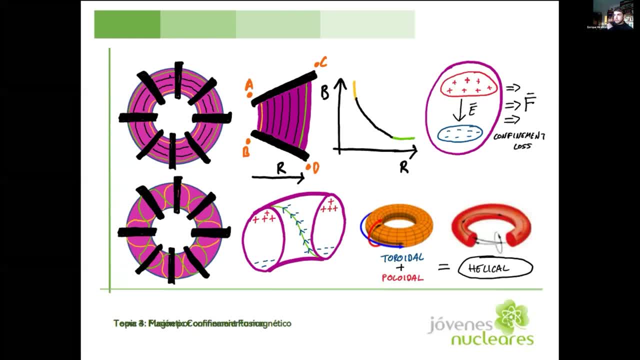 like a torus, like this. it was a good idea. actually. this is starts to look more like a modern reactor, but still has its problems. and if we take a section here, we see that the distance between a and b is smaller than the distance between c and d, so the magnetic field of the orange line is 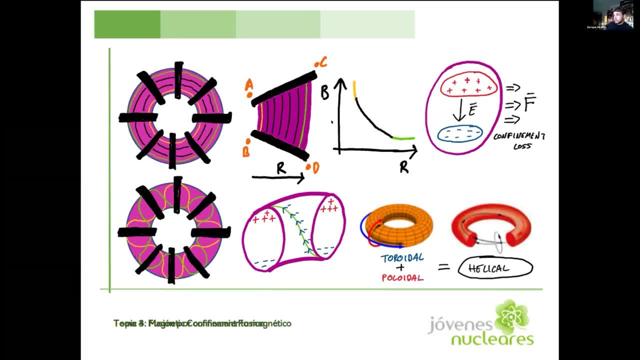 greater than the magnetic field of the green line, and the consequence of this is that, um, the positive charged particles will move in a opposite direction, um to the um of the negative charged particles, so we have some kind of charge separation and we, when we have a region of the 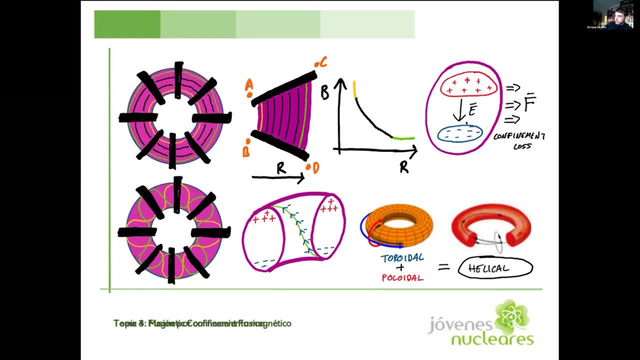 space that is positively charged and the region of the space that is negatively charged. we have a electric field between these two regions and this electric field is what is going to do, is it's going to push both particles towards the um, towards outside the reactor, so we'll have some confinement loss. so they had to figure out how to um short-circuit. 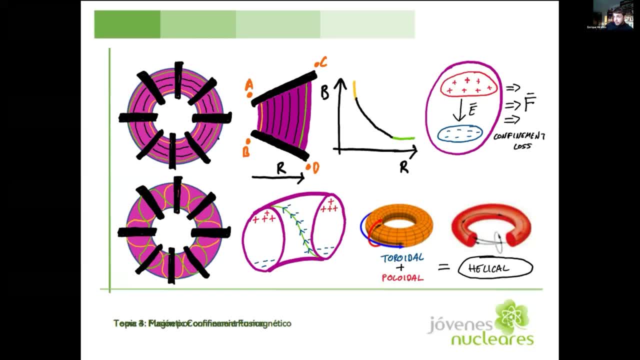 this electric um electric field, and the idea is that we need we need to eliminate um the fact that there are field lines that are stronger than others. so we need to make this orange um field line to be as as strong as the um, as the green one. so we need to make these field lines to drive a trajectory like this. 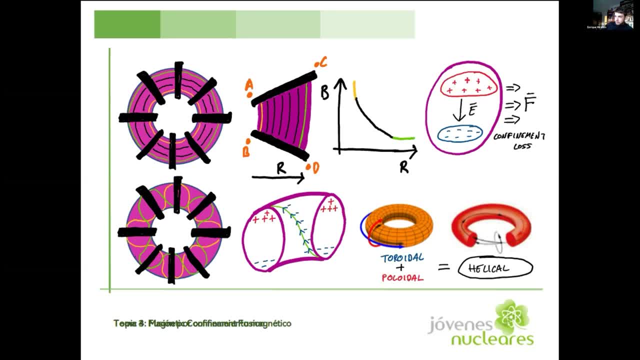 but also up and down. so this, this field line, this trajectory is called helical. this is a helical field line and what it does essentially is that it connects the a bottom part of the of the um reactor with the upper part of the reactor and the electrons. 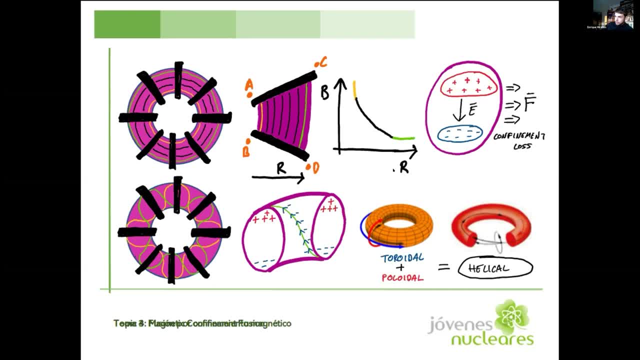 because they are much lighter than ions, they will accelerate a different way and they will accelerate towards the upper region of the space, and then they will short circuit, they will shield this electric field, And this is how the two modern concepts of magnetic confinement fusion were. 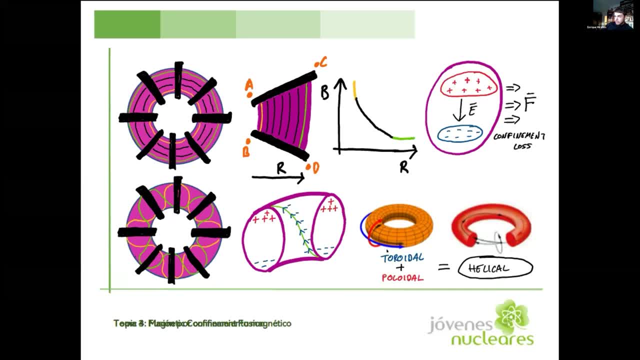 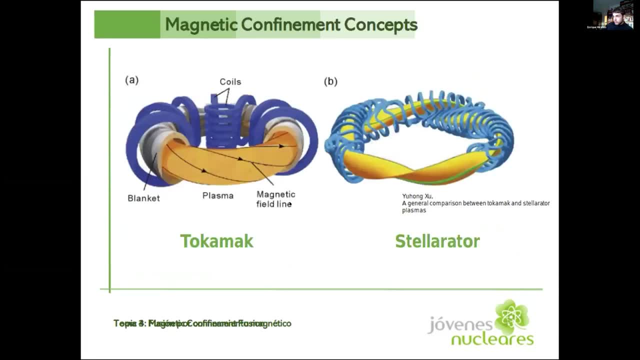 born because they essentially differ on how the helical magnetic field is generated. In the case of the tokamak, we have a central solenoid in the middle and this central solenoid is going to drive a current through the plasma and this current in the plasma is going to generate a 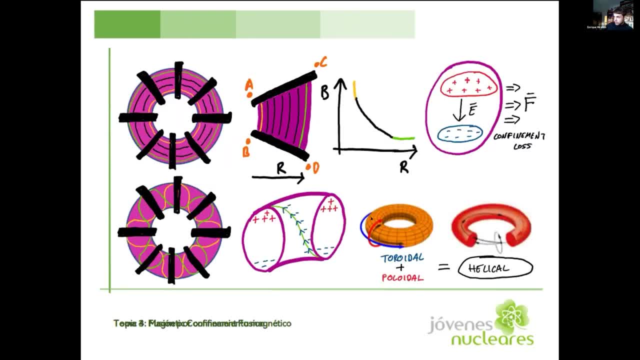 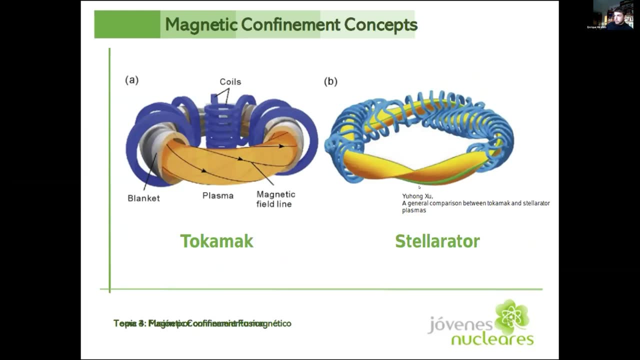 polyoidal magnetic field like this one. So it's going to make to generate a magnetic field that is going to wrap the torus like this. it's like the red line, And the way the scleriater generates this helical, produces this helical magnetic field, is naturally because they 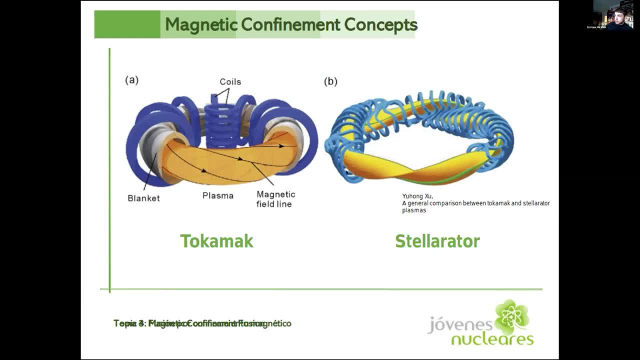 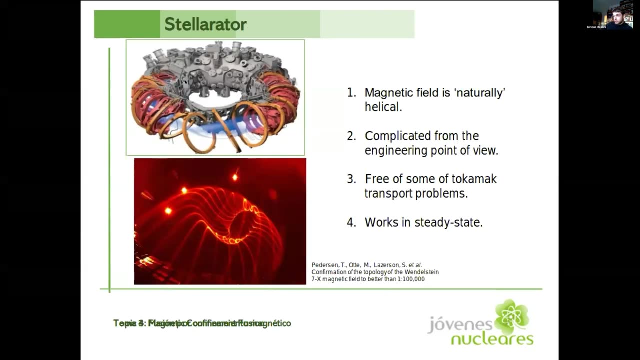 shape the magnets like this in a non-axis, symmetrical way to naturally generate a magnetic field that is helical itself. So this is Wendelstein's 7x. this is one scleriater in Greifswald, Germany, And, as I said, magnetic field in the scleriators are naturally helical because of the shape of the 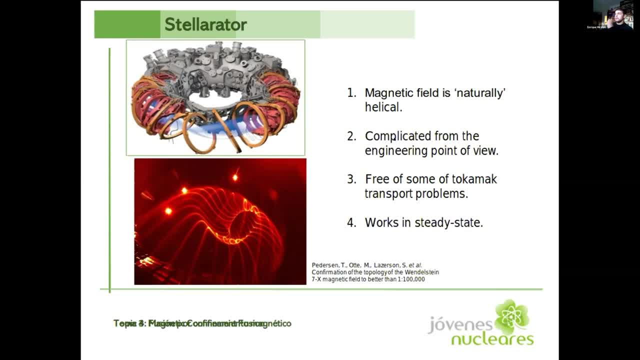 of the magnets. It's complicated. from the engineering point of view, which is manufacturing these magnets, it's very complicated. They have to be very precise and they have some other advantages regarding physics. For example, they are free from some of the tokamak transport problems relating particles and heat And they also work in steady. 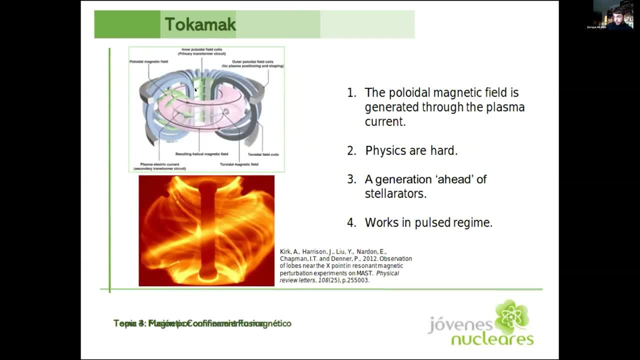 state because we don't in scleriators, we don't have this central solenoid To make the polyoidal field. we need to ramp up a current through the central solenoid and we cannot ramp it indefinitely. We have to stop at some point. So that's why tokamaks work in a pulse regime. 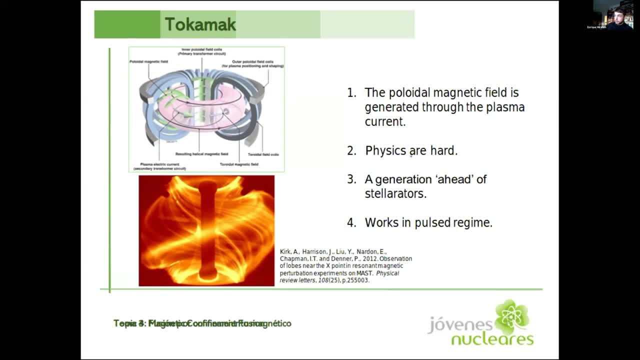 But it's much easier to build a tokamak than a scleriater, And the problem is that physics are harder for tokamaks. We say that tokamaks are a generation ahead of scleriators because we have built many more tokamaks than scleriators, So we know more about tokamak. 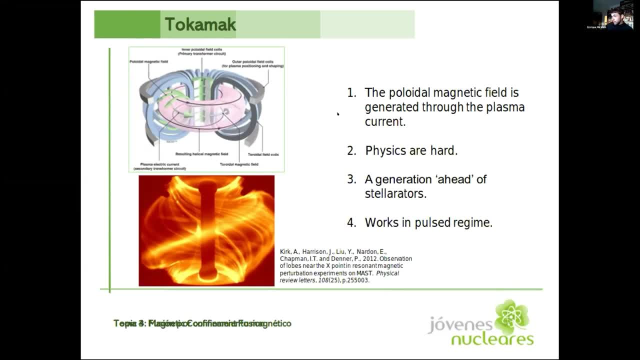 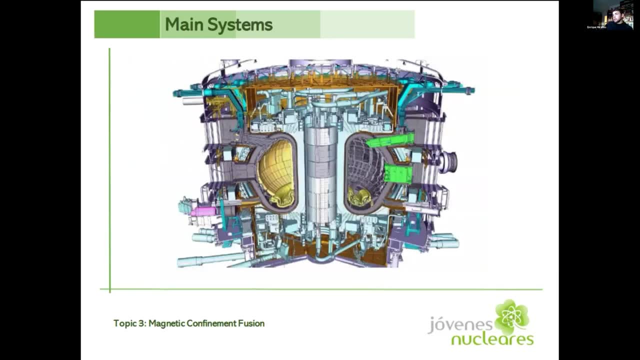 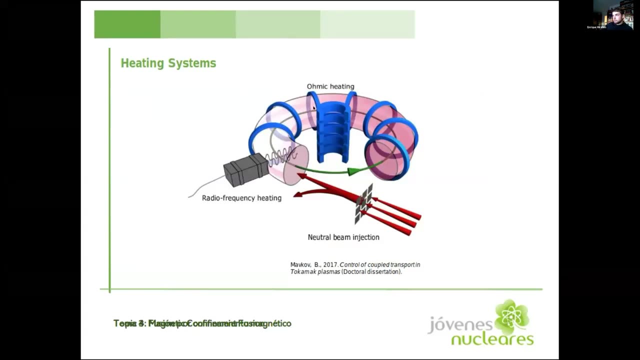 construction than scleriator construction, And this is MAST in the in the UK. So what are the main systems of a fusion reactor? I want to talk first about the heating systems. How do we heat the plasma? There are three main methods. Two of them are common for. 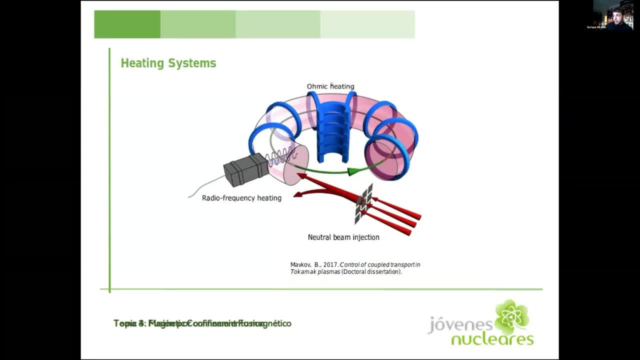 tokamaks and steliatores. But the atomic heating is not available. because, if we're still, because the ohmic heating is basically the plasma current, The current that goes through the plasma is the one that heats the plasma itself, because of the conduction losses, right? 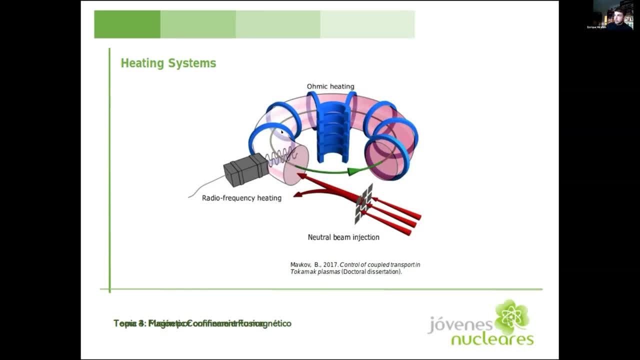 We have some resistance in the plasma and it's the Joule effect basically. But because in the oscillators wouldn't have this central solenoid and this plasma current, then wouldn't have ohmic heating. But then radio frequency heating and neutral beam injection are common. 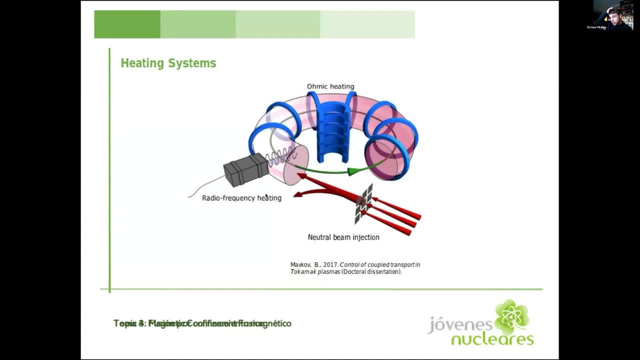 So in the case of radio frequency heating, what we do is we drive microwave radiation that has the same frequency as the electrons in the plasma or ions in the plasma, and then we excite those particles And also we have neutral beam injection. What we do here is basically we inject. 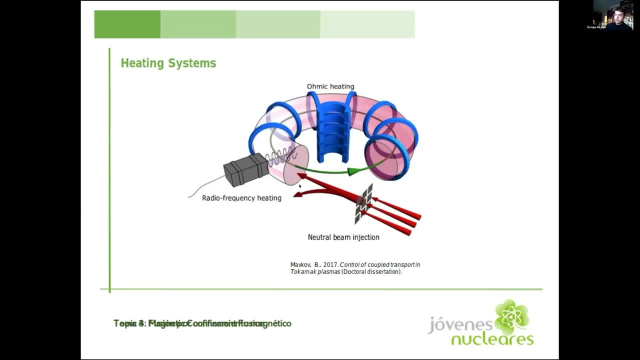 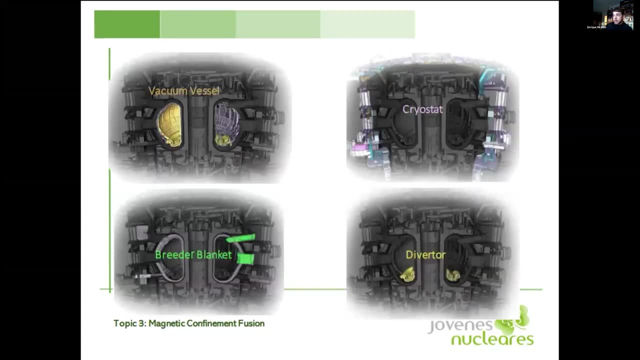 very high energy particles, neutral particles, because we cannot inject charged particles Because of the magnetic field. So when we inject these neutral particles they collide with the particles in the plasma and then they hit the plasma. What else we have? So the vacuum vessel is where the plasma 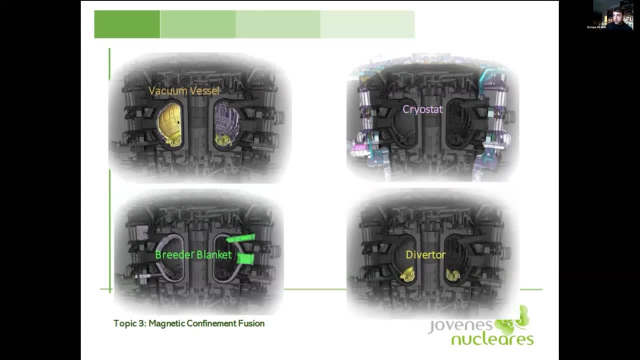 is going to be generated, It needs to be in vacuum and also very clean, because any impurity that we might have inside is going to make some loss of energy confinement time. We need to. We need to have these vacuum vessels very clean from impurities because we don't want any unwanted radiation. 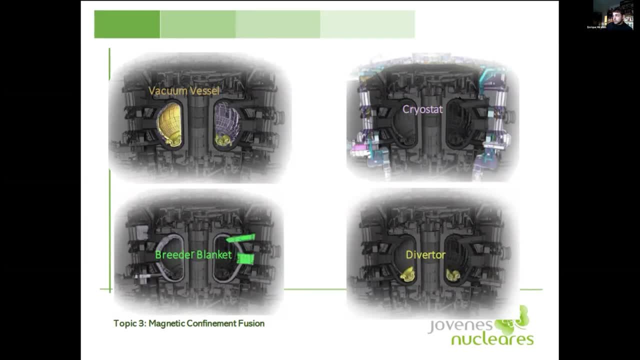 Also the cryostat. because of the magnets they operate, that with the superconducting regimes They need to be very cold So we need to cool them in the cryostat. The breather blanket. the objective of the breather blanket is to produce tritium. 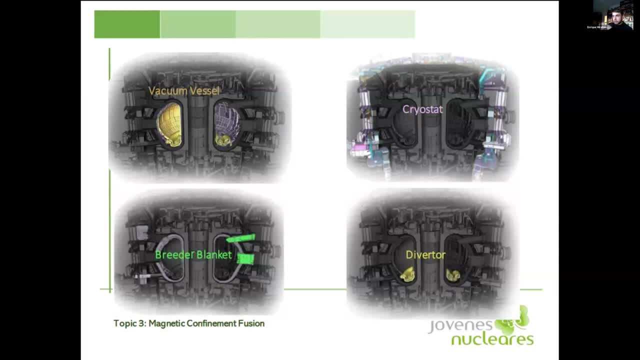 The neutrons being produced from the D2A fusion reactions, um will be absorbed by absorbed by this um breeder blanket and then they will interact. these neutrons will interact with the lithium of the blanket and we they will produce some tritium. the problem with the problem of dt fusion is that tritium is a very scarce um material. 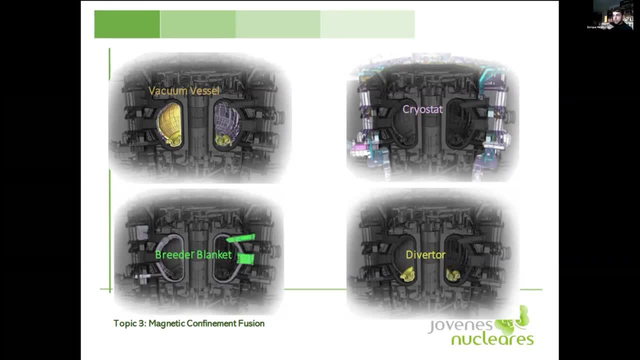 on earth, and we need to um, we need to um build, we need to create it um, and that's that's the objective of the breeder blanket. um, the deuterium is fine, we can find it in the ocean. it's not, it's not a problem, and the objective of the diverter is to remove um the excess of heat from the plasma.